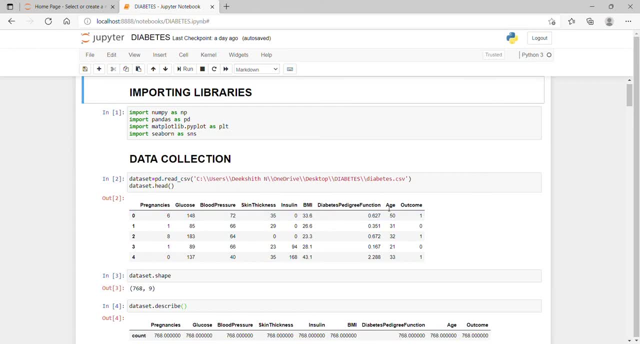 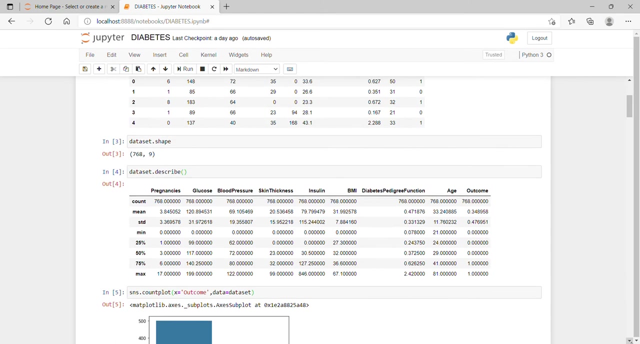 Insulin: BMI, Diabetes, Pedigree, Function, Age Outcome. In this outcome1 represents a person with diabetes and 0 represents a person with No diabetes. And here, in the 3rd step- And here we have been doing the- We have done the shape of our data set, which gives the number of rows and columns, and in the data set which we have uploaded we have 768 rows and 9 columns. and then we have been given the data set dot describe, which gives the mathematical values, like 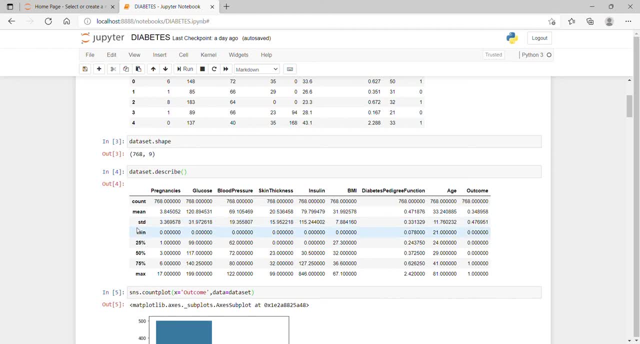 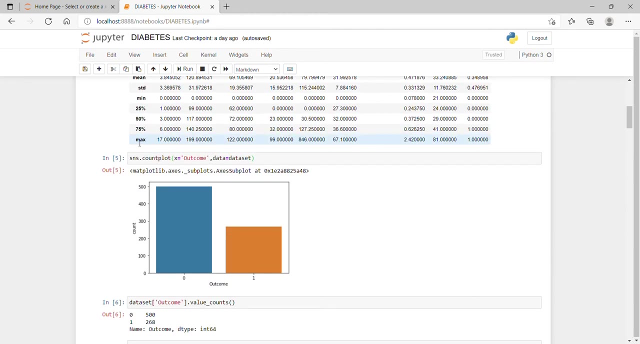 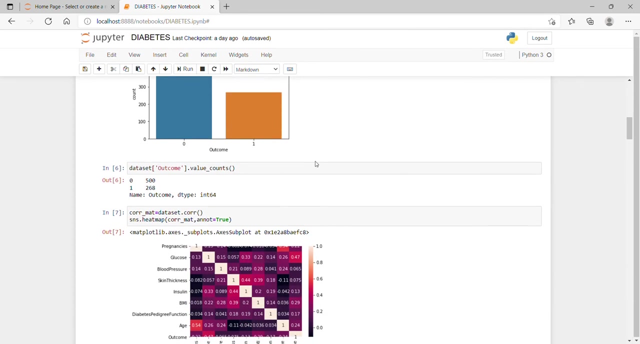 dot count mean standard deviation, minimum, 25%, quartile, 50%, quartile, 75% and maximum it will give. and then we have been plotting the graph for the outcome and the total count and we are getting the plot like this and again here, here we have been doing the total number of counts, here we: it will give the. it means here give the total. it will give the persons with number of persons with diabetes and no diabetes. by giving this, we got no. with no diabetes there are 500 people and with diabetes, there are 268 people. 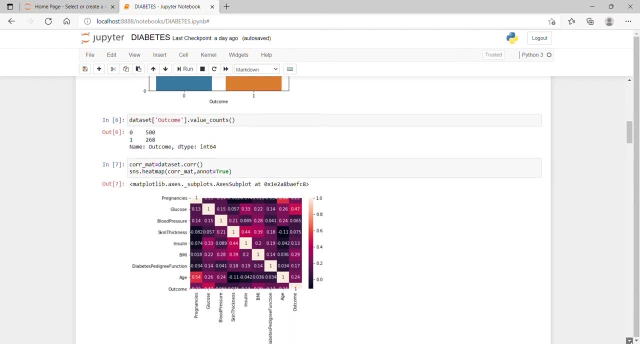 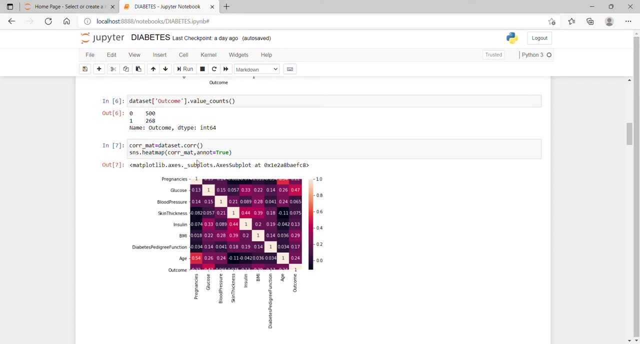 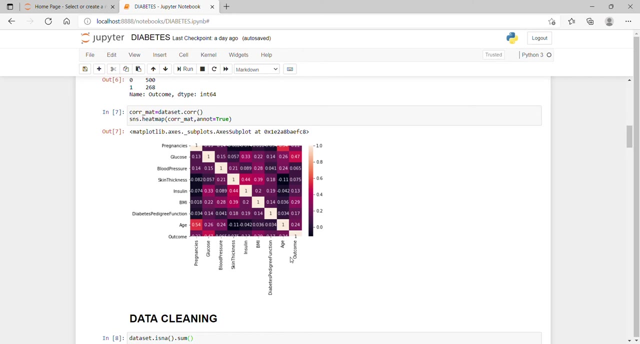 Now, here we are going to the test: returning the multiply, get the prediction data set. So if I go to my personal measurement instrument, I will get the value and the. here I will go to reference analysis and now here is the improvement It gets: reduce the clip to the reference. 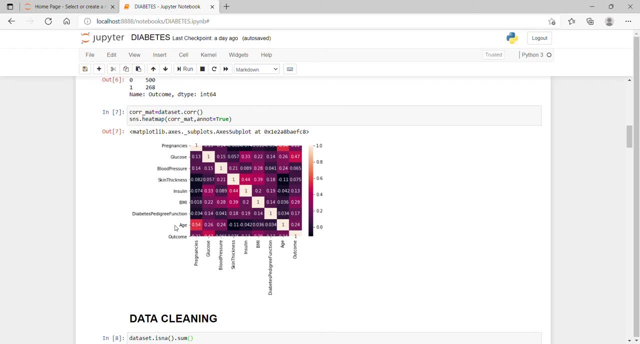 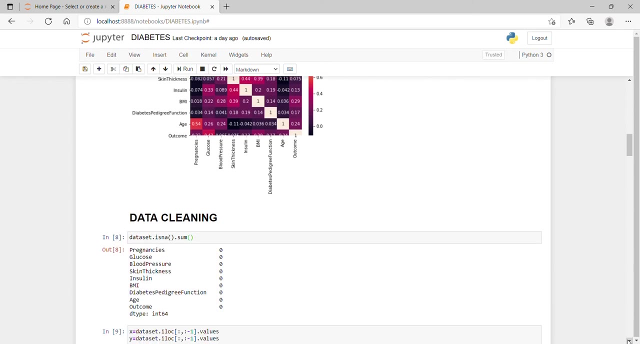 It gets, reduce the clip to the data set. and again, after going to this, we have to do the correlation matrix correlation, and it is a heat map and in this we will have this values. It means doubt, Comparing with age and glucose and comparing the outcome. and glucose is 0.47.. It is a maximum of all this way. and then here we have to clean our data. 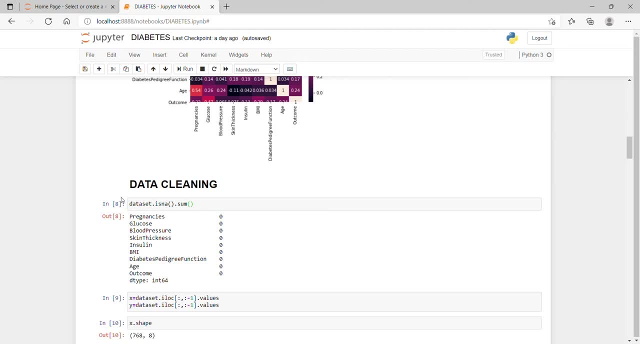 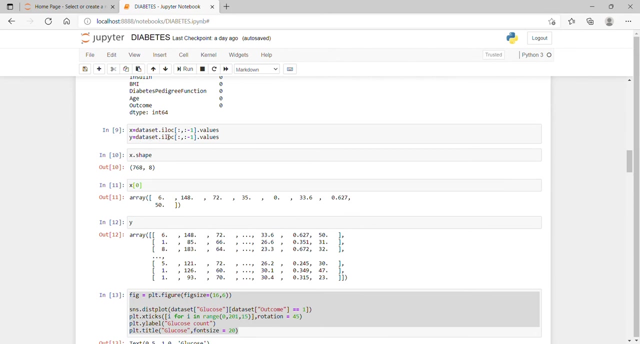 So it means, by giving this, it will show the number of columns or rows which add 0 values, which are null values. In our data set there are no null values and here and after this we have given x data set- i location and y data set- i location. 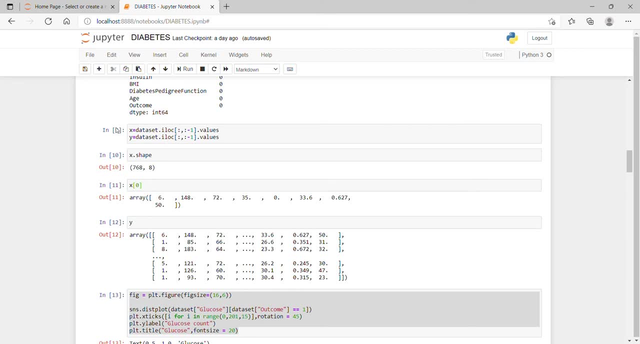 It means it will give. here we are doing the developing the. we are giving the independent values into one single array and dependent values into single array and after that we are doing the shape of the x, we are getting 1768.8 and x value and 9 value and again. 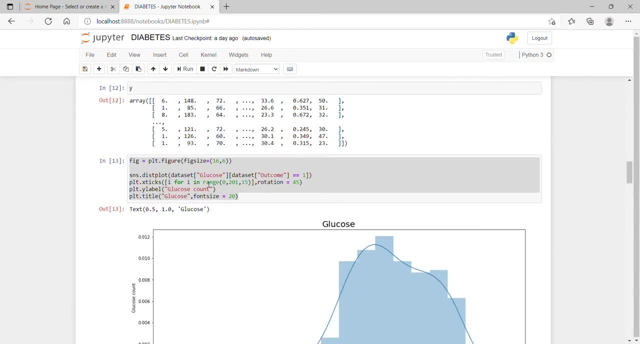 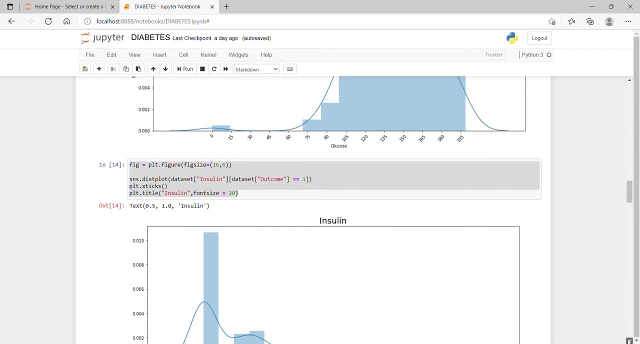 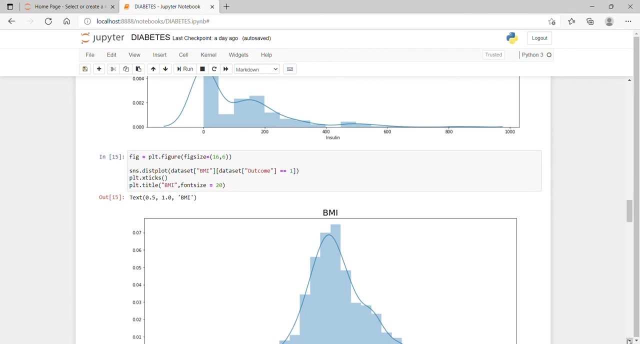 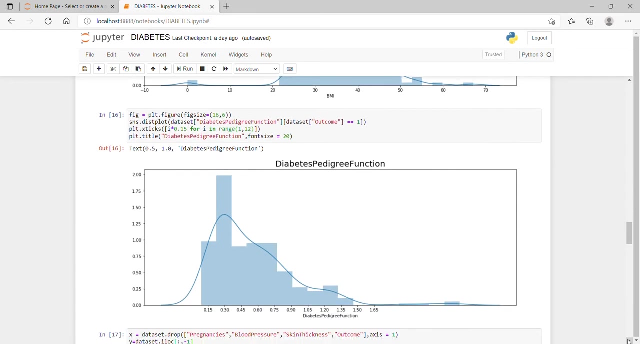 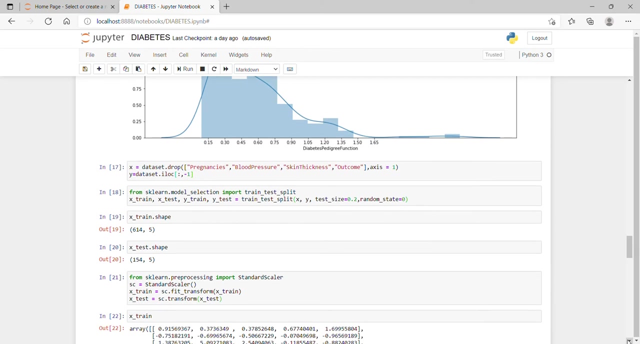 and now we are plotting the graph graphs with the glucose and outcomes in this. again, here we are plotting a graph between insulin and outcome. and here we are plotting the graph between bmi and outcome. and here we are plotting the graph between diabetes and outcome. and now, After that, here we have removing here. drop means we have to remove these four columns from our data set. 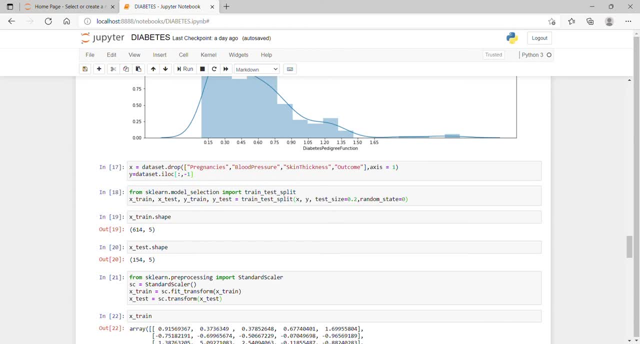 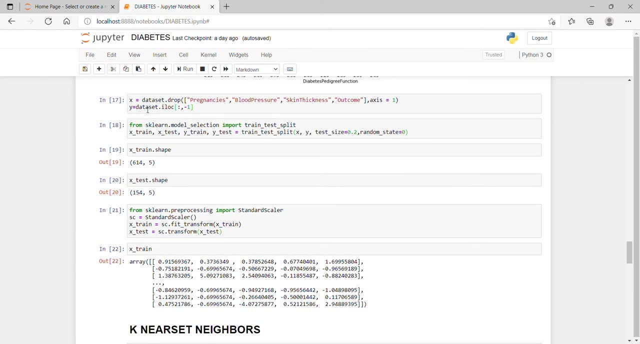 And after that we are. and after that, after removing the, after dropping the pregnancy, blood pressure, skin thickness and outcome we are giving from escalate scale and model selection. import line test split: extend y test, y train y test. 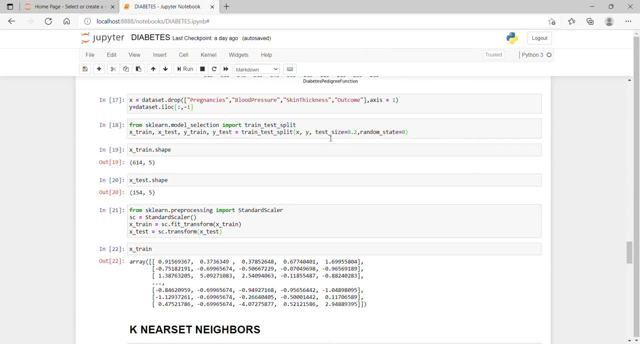 And this here test size equal to 0.2 means From our total data set, we have to do testing on 20% of the data and 80% of 80% of data we have to retrain it. 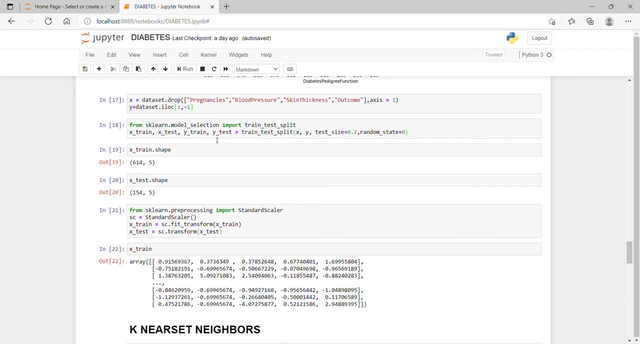 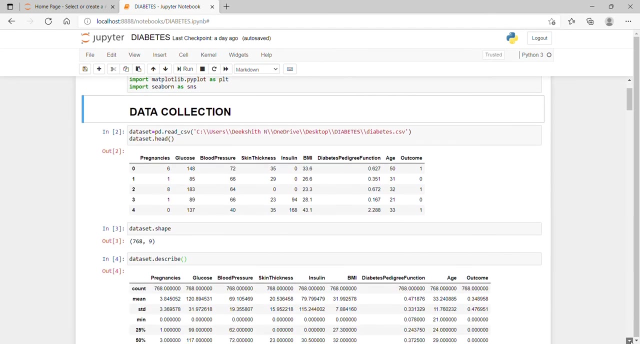 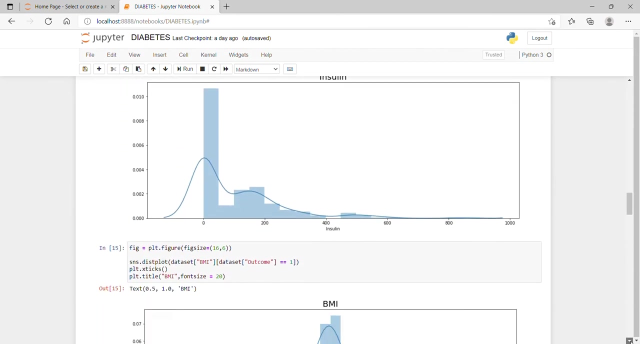 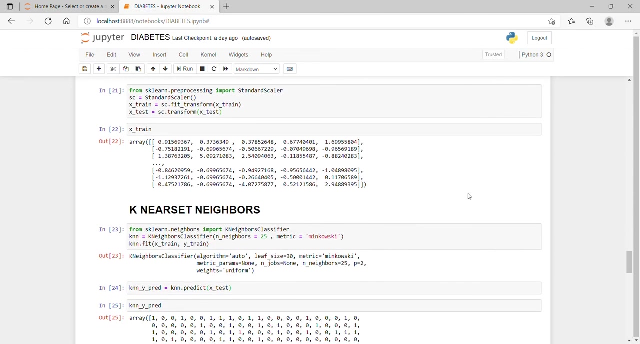 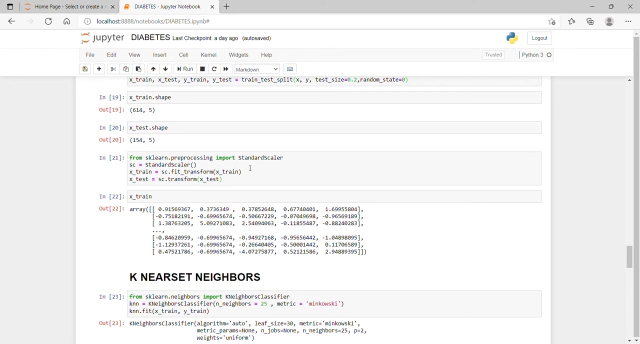 And after doing this, extend extend y, train y, test- we getting the shape 614,5 and extend step shape 154,5.. And again later, And here we are doing the future scaling here. standard scalar means it is to standardize the independent futures present in the data in a fixed range. 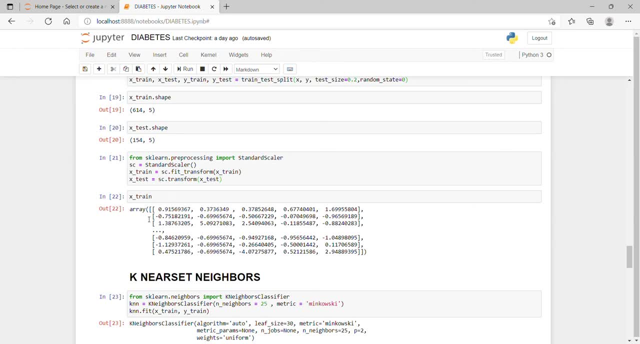 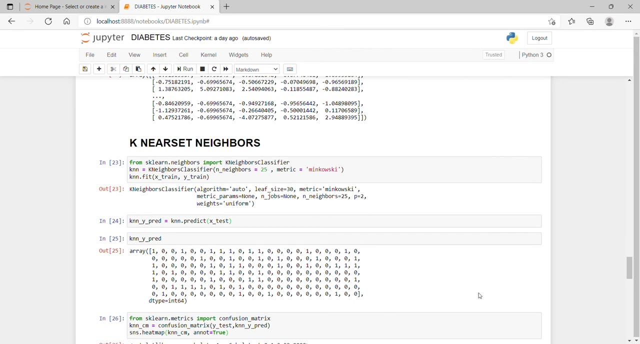 It means it will make all the values to 0.2.. And once and here we are giving, after that we are giving the extend, and now we are. and now we are doing the K nearest neighbors algorithm, Here from a scale and as neighbors import, K neighbors classifier KNN, K neighbors classifier and neighbors equal to 25 metric mini cost and we have to fit the extend and y train. 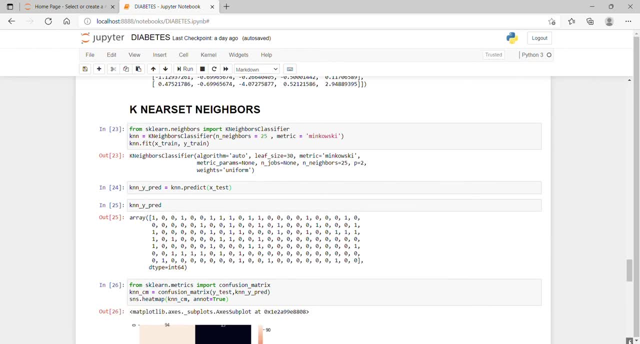 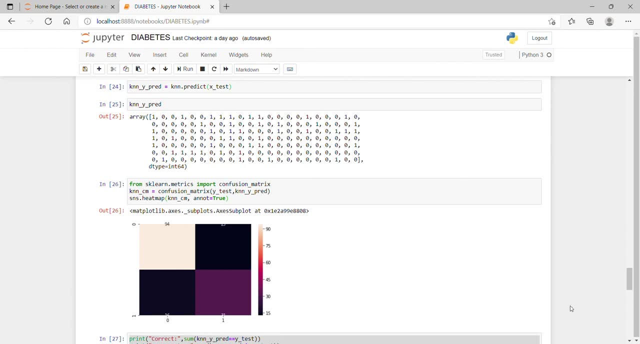 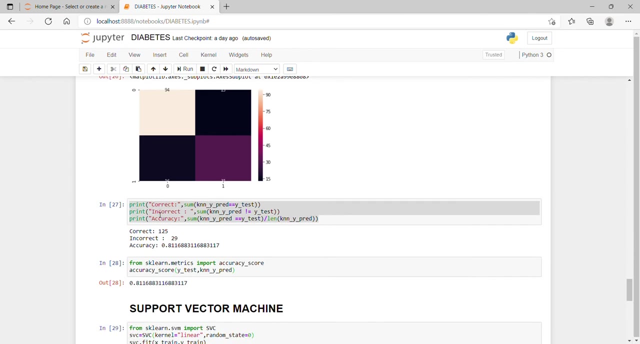 And after that we have to predict, And after that we are drawing the confusion matrix For the KNN KNN algorithm And after this we are getting the we have to print accuracy in in current and current values. 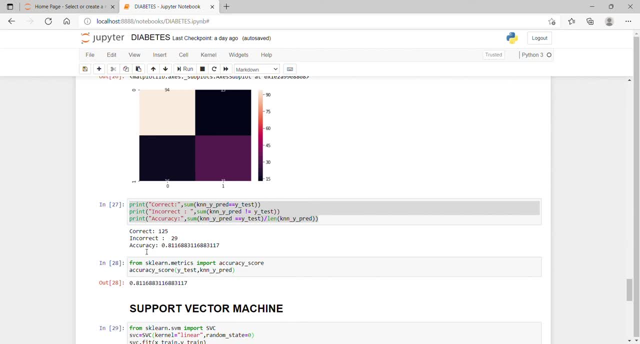 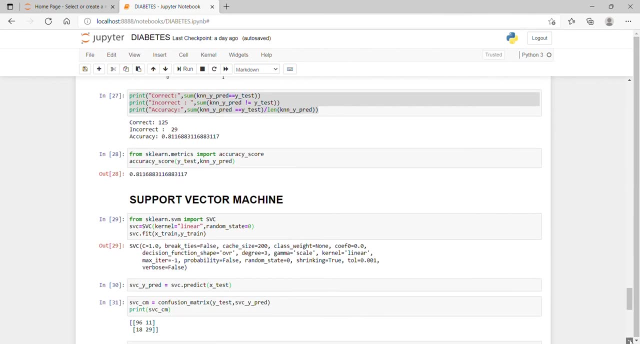 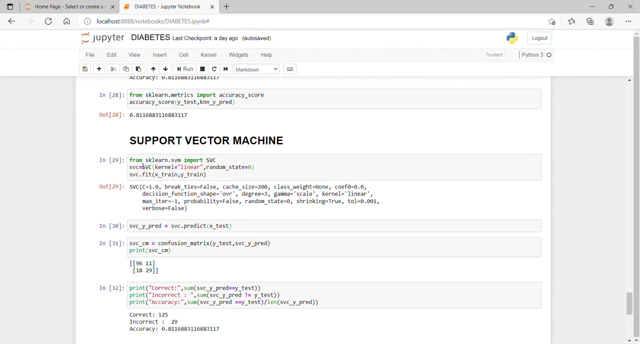 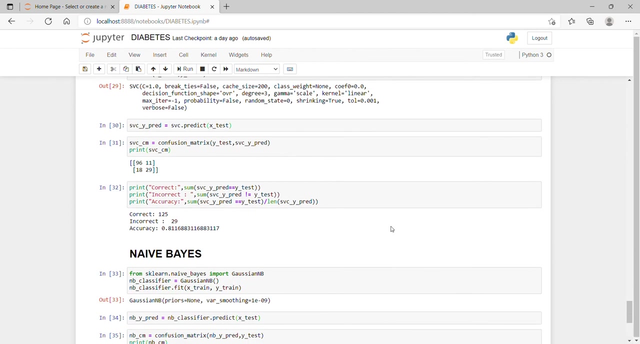 For current. we are getting 125, incorrect, 29, and accuracy 81% And And And From again, we are doing one more algorithm: support vector machine. here we are. we are doing the SVM support vector machine algorithm. here we are in the same, the same process, here, confusion matrix, and we are printing correct, incorrect, accuracy and we and the same thing: we are getting 81% of the accuracy values. 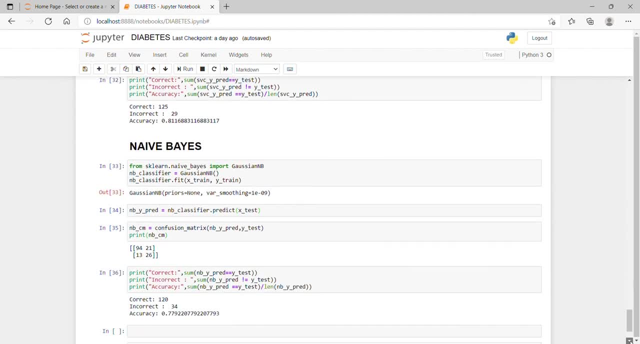 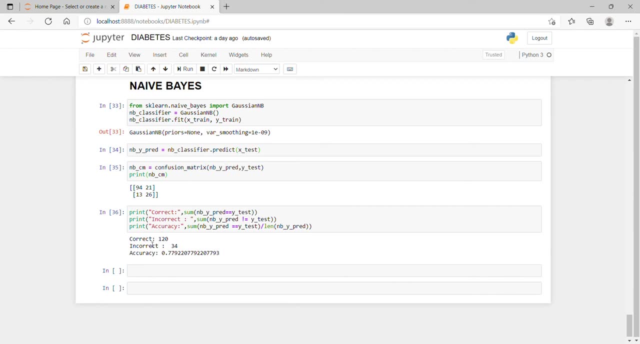 While using SVM And after that Navi base algorithm, And here also confusion, matrix accuracy and everything, And we we have got 77% accuracy With this 3 algorithm, with this 3 algorithms.